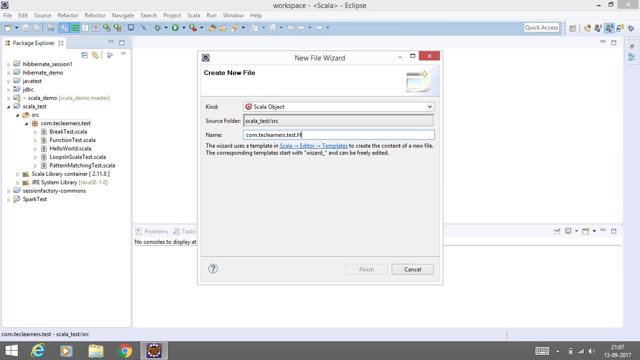 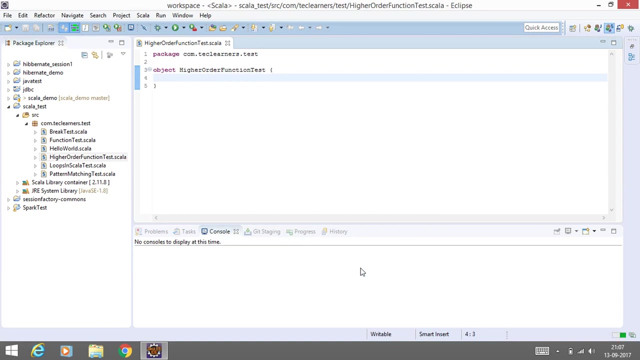 let it be function test. okay, so my program will start from min. so first of all I'll color function as a parameter. say, let's say 25 from multi. so here the multiply by two years. another function. I'm passing a function as parameter, so I'll have to do one thing. I'll have 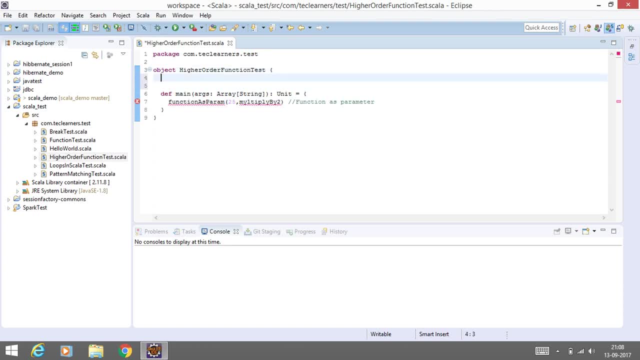 to make a function here function as pattern, do it first, then another function: multiply by 2. yes, I will give one input to this function and it will return int. now, just make it a now, now, now, now, now, inside this what I will do. I will according to the main function. 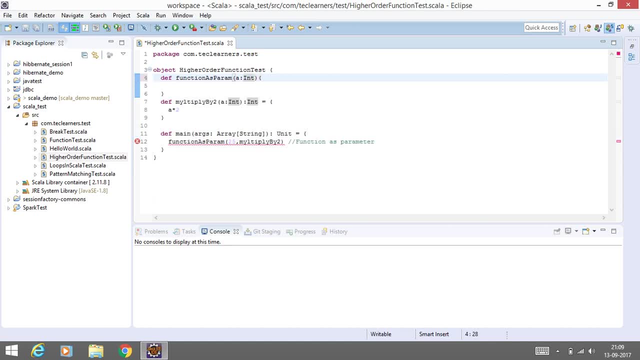 I will have to pass an integer type of data and another is a function which will will return int, and this is going to be int, int, int, passing a function as a parameter in a function, and I will provide the input to this function. yes, now you just try to understand this now, here, here, and taking 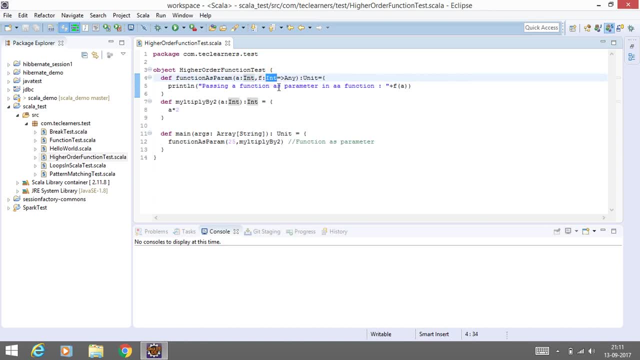 the input of integer type and returning any type of data here here. if you sorry, I have not told you that about anonymous function. what is anonymous function? anonymous function is a function that has no name, but it works as a function. now, here this can be an anonymous function which doesn't have a 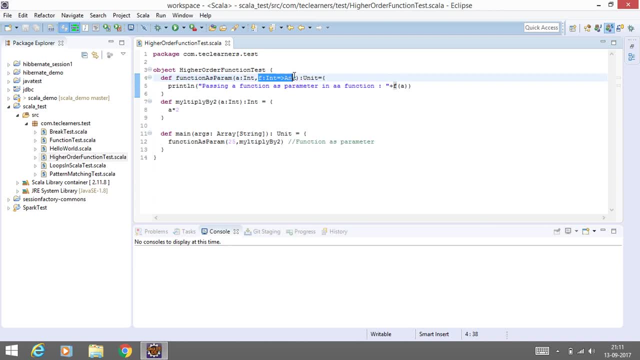 function body and it doesn't have a name, but it works as a function. you can create an anonymous function by either using rocket operator- this is an rocket operator- or by using underscore. I also give you an example of function anonymous function. okay, let me first show you the example of an anonymous function. so let's say: 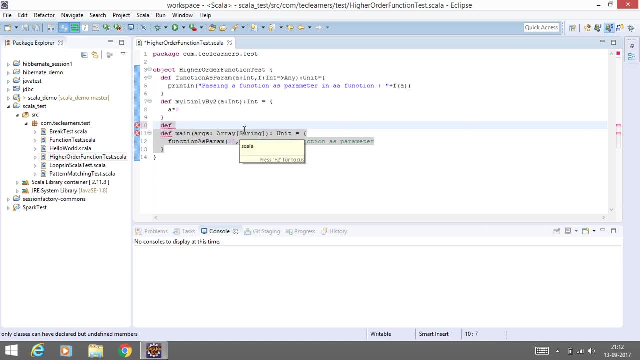 after then I will come to this path. okay, anonymous function. if anonymous, I'll use both the rocket operator and underscore for creating an anonymous function. so first let's start with rocket operator and let's take two like integer and build also integer. now this anonymous function will take two. 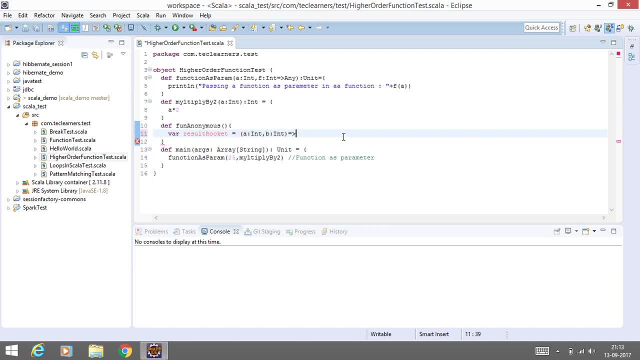 input of integer type and what it will do. it will return the addition of but there and puts ok, now I'll try with the underscore reasoned in the skirt. now we can also access this by using underscore, so in case of this underscore we can write it like this: integer class and the scroll integer. now you can. 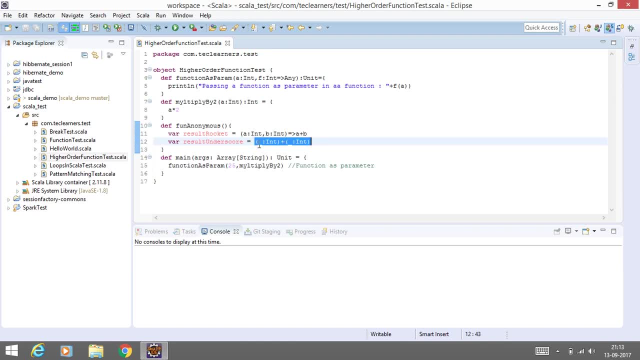 directly return the addition of that input. now, this is an anonymous function input. this is the anonymous function input, so both the inputs will be added and the result is third to the declared variable. yes, so let me call this. I'm calling this inside. suppose I have to print the value of anonymous function by? 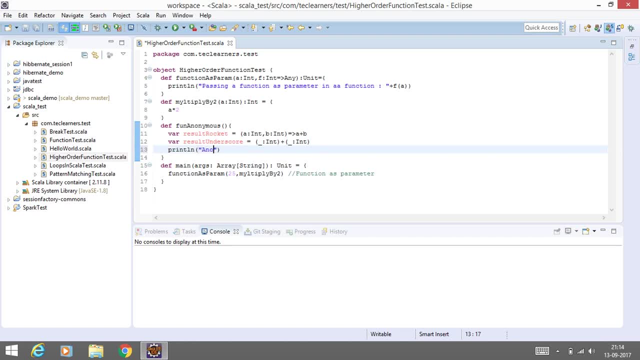 using both operators: anonymous function. anonymous function by using a rocket operator. by using rocket, a result: rocket. why is it important? is because here there are, yeah, and I'm giving 10 equals steps to MYMBODY and I'm giving 2 inputs to this: 10 and 20, the same thing. 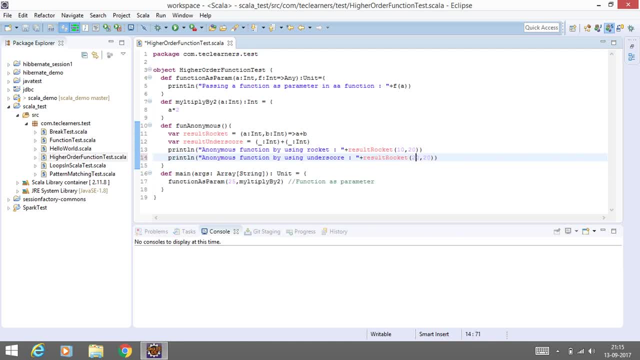 function using underscore. now let's make it 20 and 30. now I'll, Windows will open with Jest for such property. I'll, Windows will open with Jest for such property, just as function. and then the math: anomalous, sorry, like this, sorry, I'm kidding. and then the month: yes, now I. 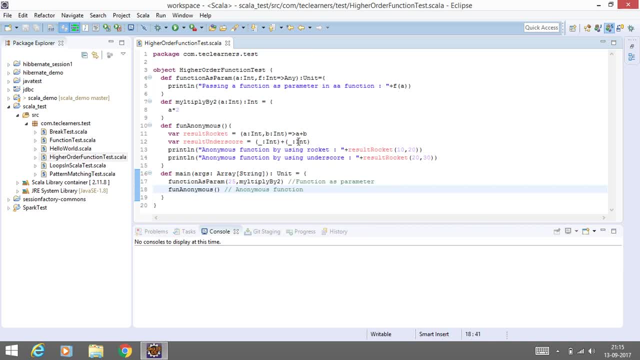 announced function. so here you can have some idea about what is an animus function. that's what I have used here. so this function will take an integer type of data like this and it will return any type of data and it will do operation that will return any type of data. so, as 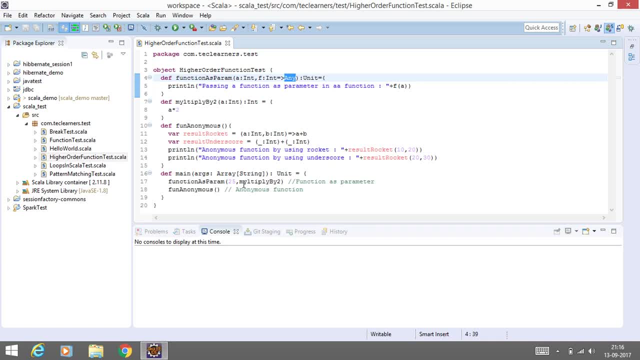 expected and I here I have put 25 and this value will be passed to here and here it will become 25. now I'm taking the function as parameter here, so what it will do. now this function will operate on a data which is of integer type, which is in. 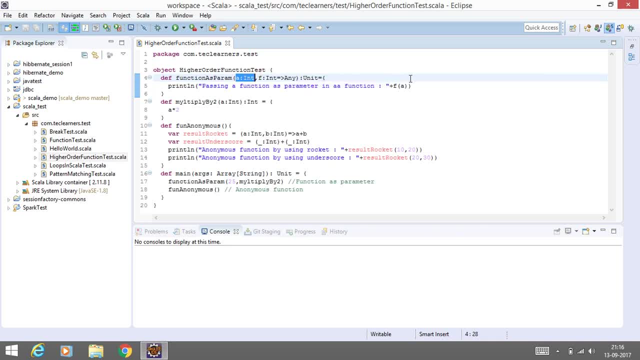 which is coming as input here and it will be passed here like 25. now this, as this is called here and now 25 will come inside this and, as expected, it should be multiplied by 2. so our answer to come 50. so let's see this. 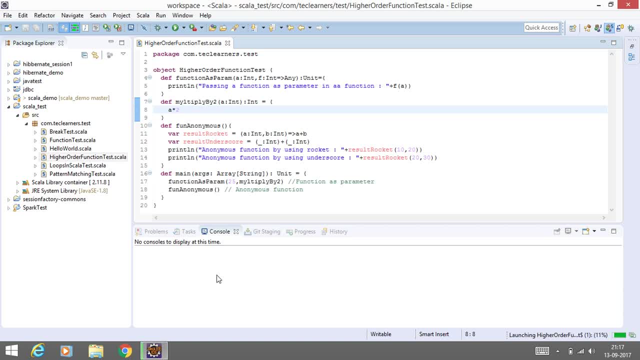 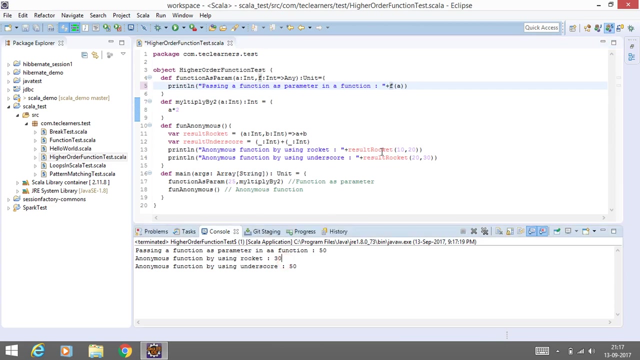 you, you, you, you, PASSING FUNCTIONS, now passing functions as function, as parameter. in a function it comes 50, as expected. now in this, an animus function, by using rocket operator, we perform some addition operation here and printing, printing that value and it is 10 plus 20. 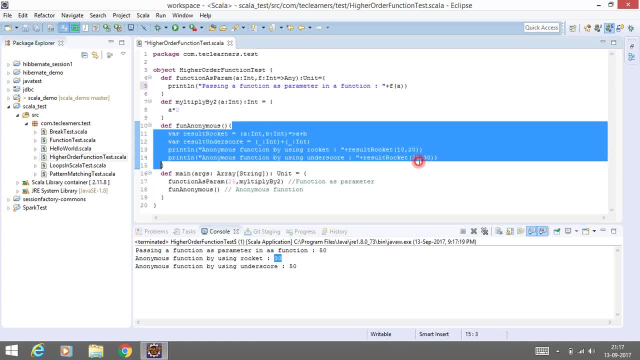 equal to 30. yes, we got it when 20 plus 30 equal to 50, and also, we got it. so next thing. so these are some of the concept. now I'll go to different. and so like function cutting, now function carrying is a technique of transferring of a. 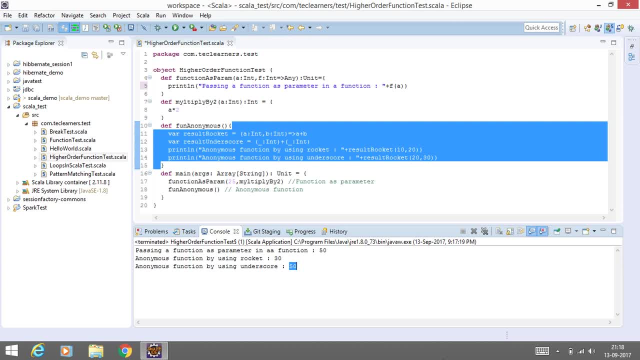 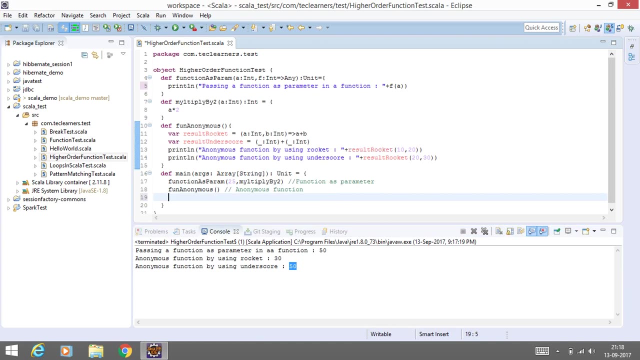 function that the text multiple arguments and it makes into a function that takes a single argument. so it's a basically a concept of reducing that answer and when I'll show you the, the practical example, that you'll get some idea. so let's make a program and make. 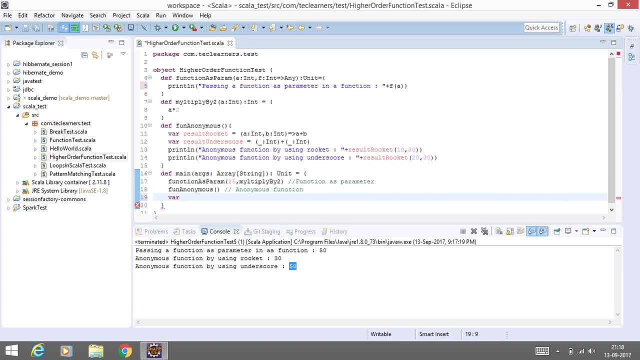 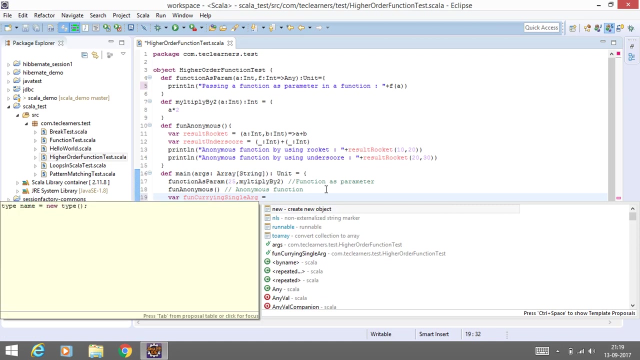 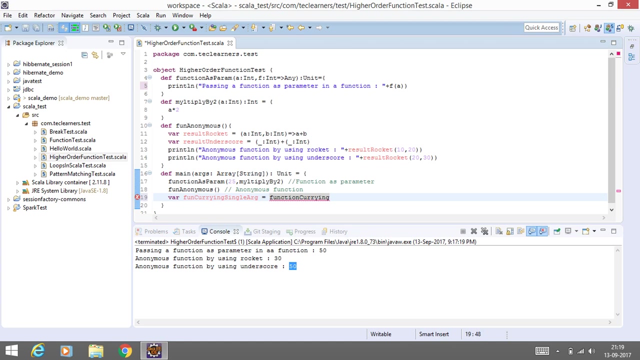 care of variable like what, what, what, what, let's say function, fun, current, go, you'll get some idea. so let's make a argument and I'll show you how you can make it. um, let's say, I'll make the name as function carrying, function, add so and and be of also having and so so. 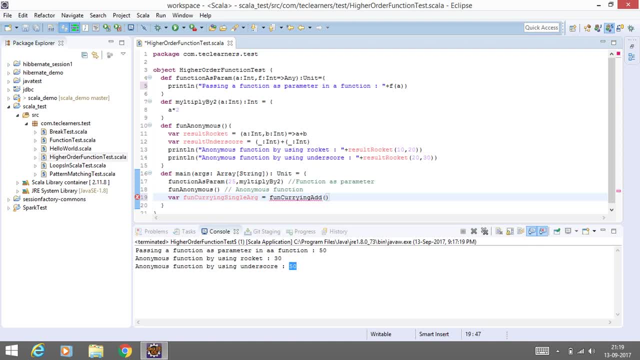 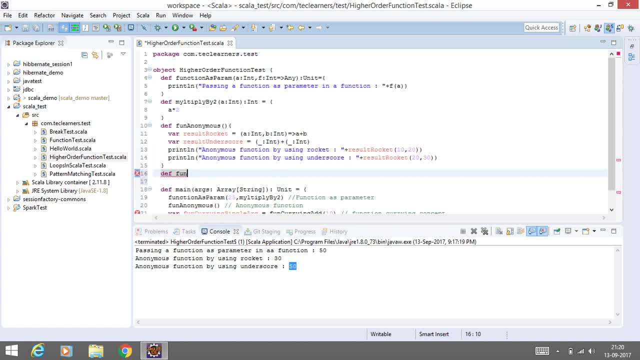 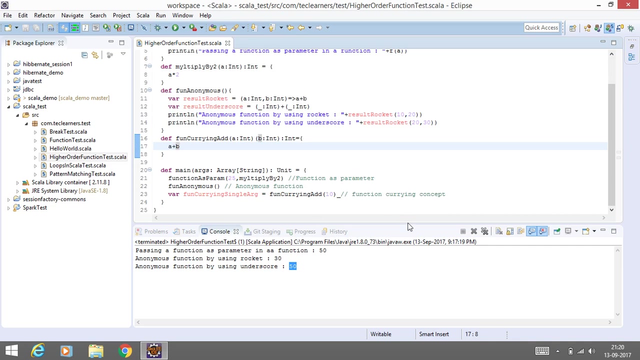 mmm, so we have 10 here and we have mmm. so we have 10 here and we have mmm. so we have 10 here and we have and, and it will return in type of data and be now and the function concept. why I'll do, I'll make another variable result. 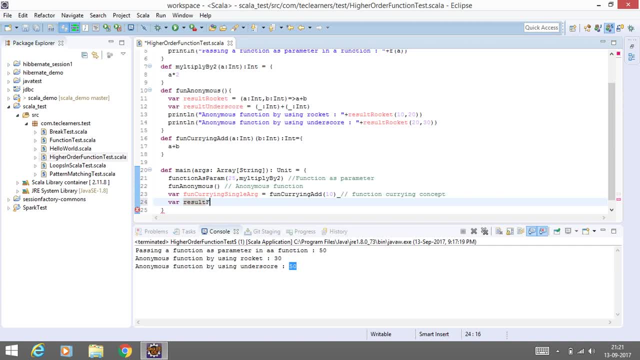 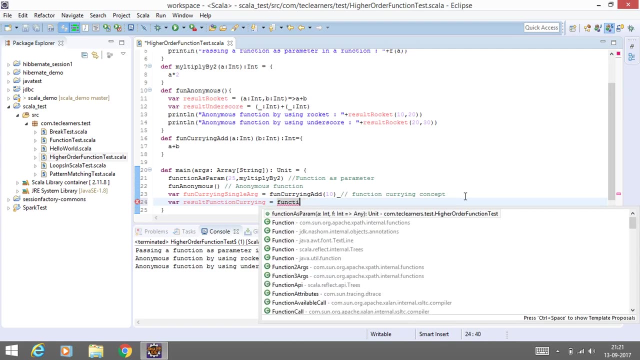 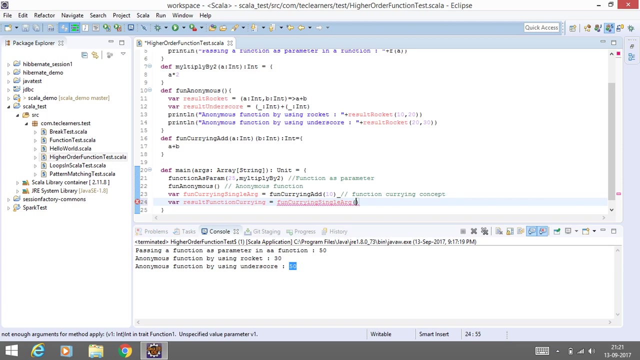 and of function current, current, and I'll pass the function current single argument from current single argument and I'll pass another variable. now I'll print into them: function current going result: function guy. yes, now just try to understand. so what I did. I do as I've told you, that function. 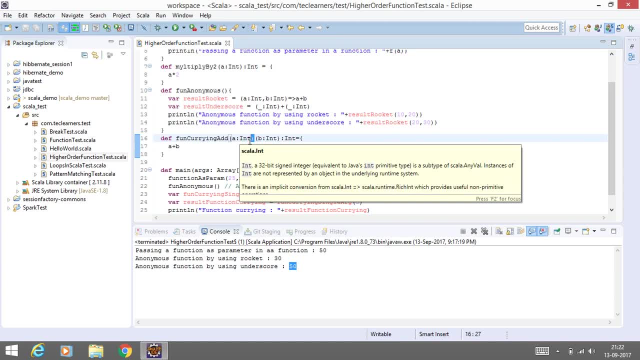 current is the technique of transferring the function that takes multiple arguments into a function that takes a single argument. so here I have taken single argument here like 10, and I created a variable function- current single argument- and I create another variable and I pass that function- current single. 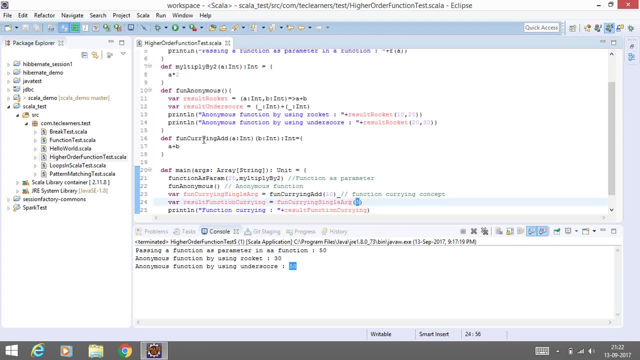 argument and passed some argument 5. so in function- current element function- current add function, I made two inputs, a and b, and here I have performed an addition operation. here you can see I have taken just one value for a function add, it is 10. and once again, before printing the final, 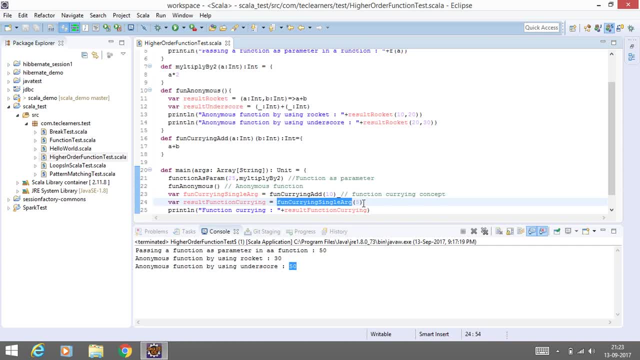 result. I put the value of another parameter in the value in the result of the previous parameter and I should get the result. now let's say yes, you can see, function current is 15. I'm getting the result as 15, which is expected, and I got. 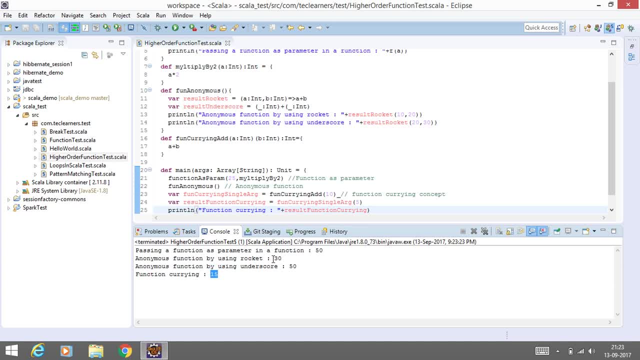 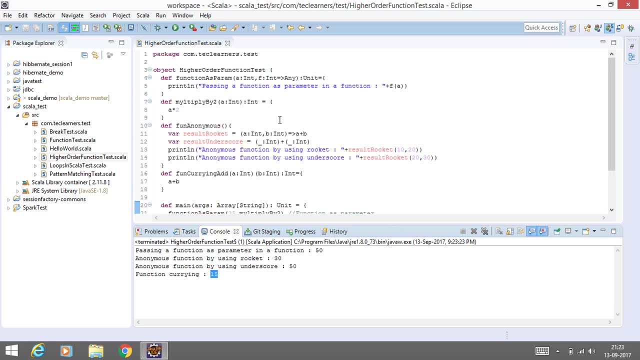 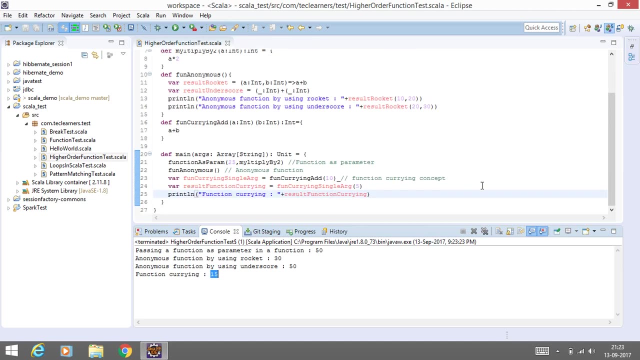 that. so it was the thing now I'm going to do is I'm going to do the same thing now. I have covered an anonymous function, function as a parameter, function, current. now let's come to another concept: function composition. let's say: first of all, let me make a function. 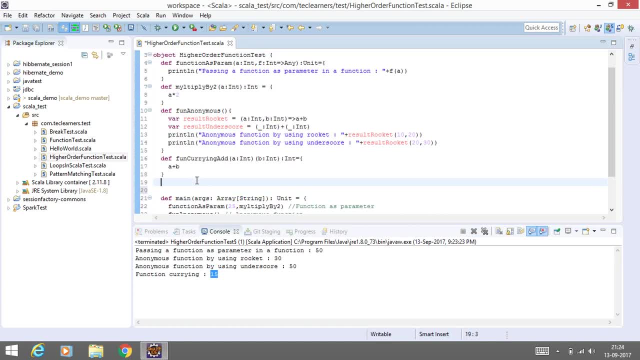 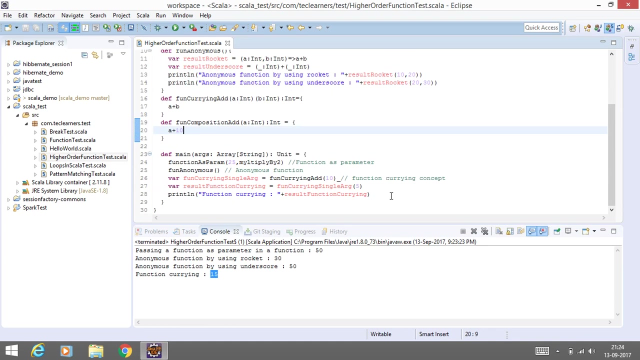 first function composition, and I'm going to call it a plus. let's attend now how to count a plus. let's attend now how to count our let's and make available recent our let's and make available recent our let's and make available recent composition. function composition and. 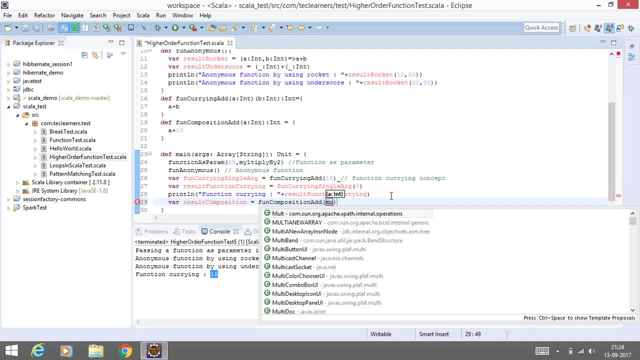 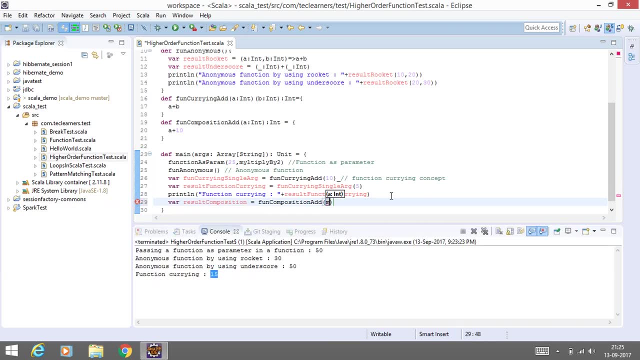 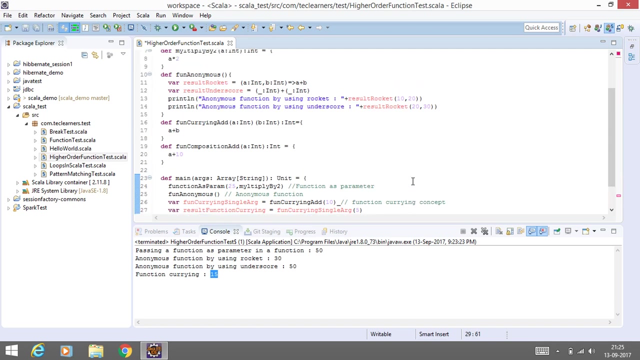 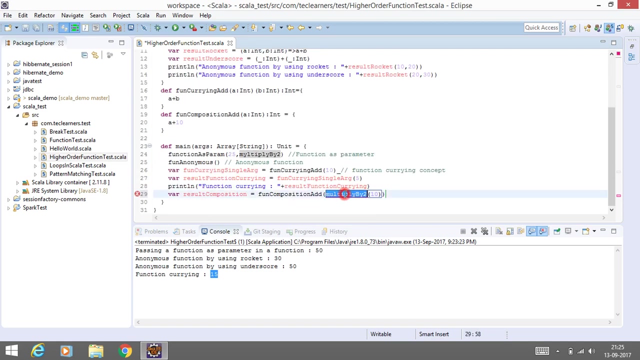 let's multi. sorry, I think it was multiplied by 2.. yes, now this has become function composition composition. so I will print the result of the function composition println. now the function composition add. so as a composition. yes, now let's see what is the answer. yes, you can say you can see here you got 30, how I have put the input of. 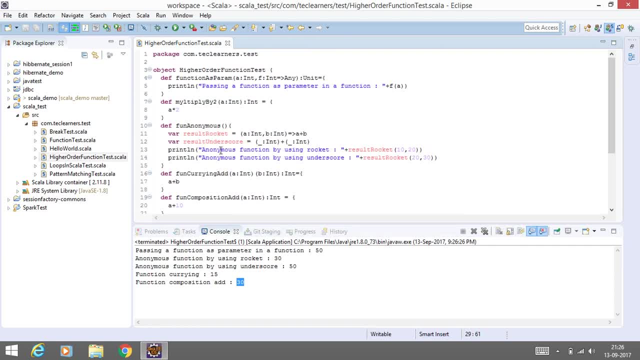 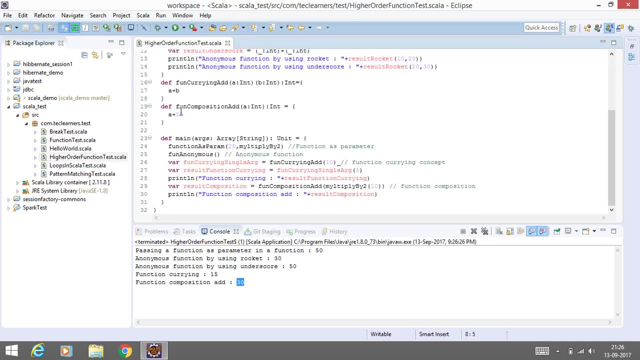 multiply by 2 as 10, 10 and what it does? it multiplies and the input by 2, so it becomes 20 and in function composition add. I have put the result of my multiply by 2, that is 20. now it is added to 10 and the final result I got is 30. so this was a 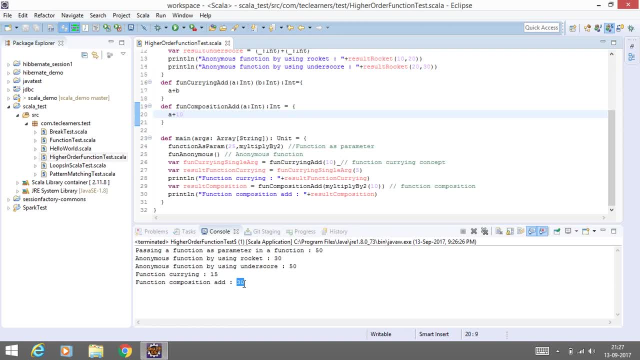 composition function- composition. now I'll show the next function how it work, okay, so first of all let me make the function instead I ah, then the end: 903 items integer. now the return times are: prosecutor. ok, uh, so in Astor and Mr as the name starts. 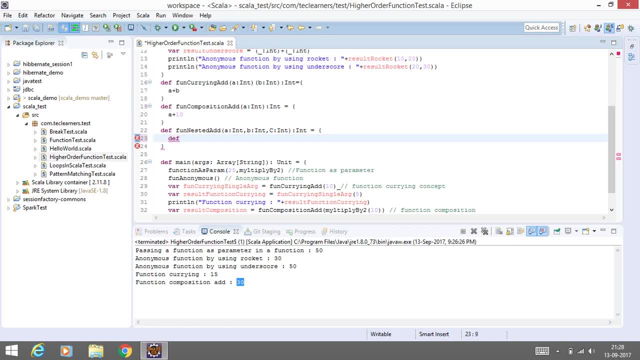 it is a nested function means the one function, another in another function. so this is the inner function which takes the value of two variable, that is, let's say, X and Y, and it also returns into the type. say it is adding this, and what? now I'll have to pass the value of X and Y. so how I'll pass it? I'll just simply: 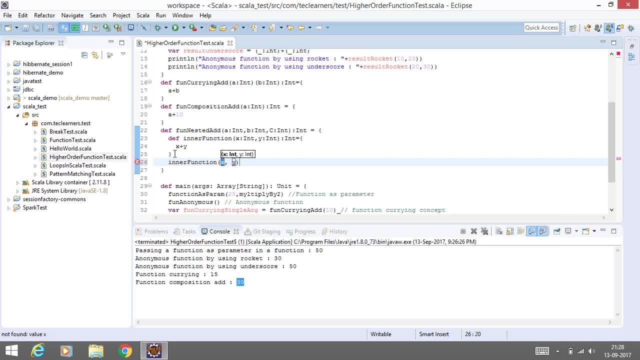 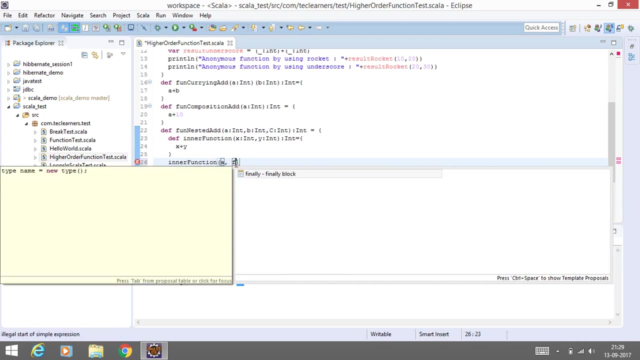 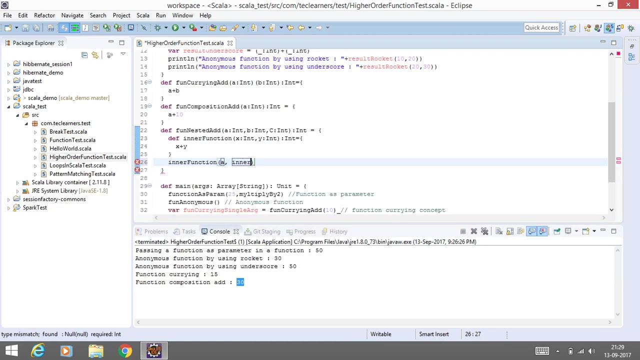 call the inner function and I'll pass a value. for value A, I'll have to perform the addition of all the input given in from nested add. so what I can do here, I can simply pass the function name here from nested enough function in the function and I'll input the value. 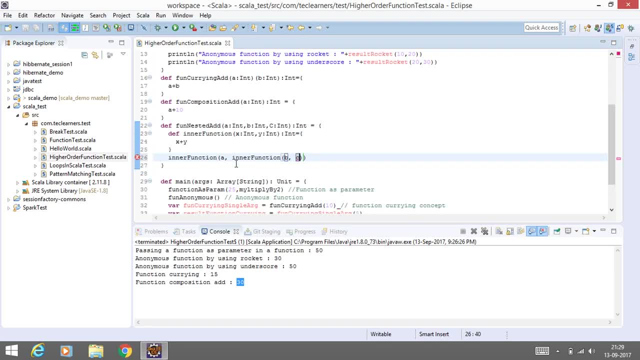 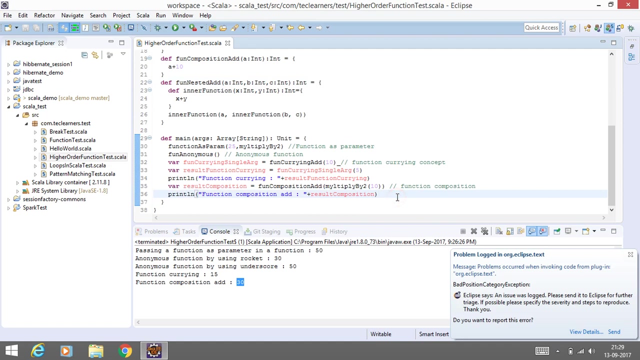 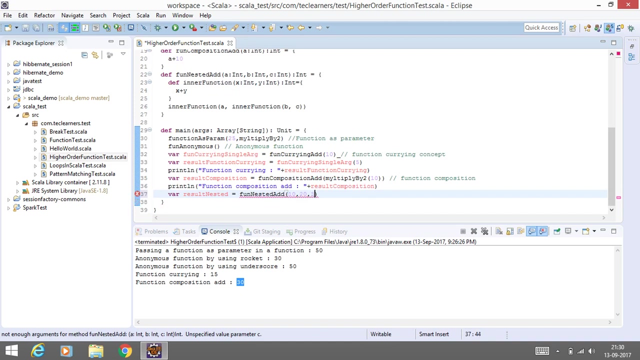 of B and C here. Now the value for B and C will be the value for X and Y. Okay, Just smalls. Yes, Now I will call it from main. Let's make a variable for result Nested Guys. I am making it so simple that you can learn it easily, So I am doing it step by step. I am putting the input for nested: add It's 10,, 20,, let's say 30. So my expected result should be 10,, 20,, 30.. 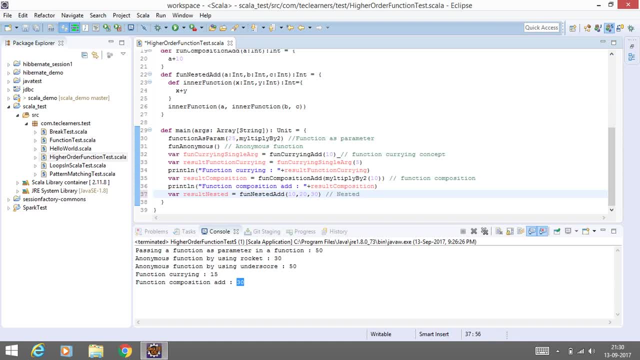 10,, 20, 30, equal to 60.. Nested function. Let's say I am getting the exit out to the not So nested function. add: All right, So nested. I am supposed to get the answer as 60.. Let's see the output is 60 or not? Yes, I am getting the output as 60.. And next thing, What's next? What's next Then? let's come to another concept, that is, you might have heard about varags in Java, So in Scala they also have the type of concept. 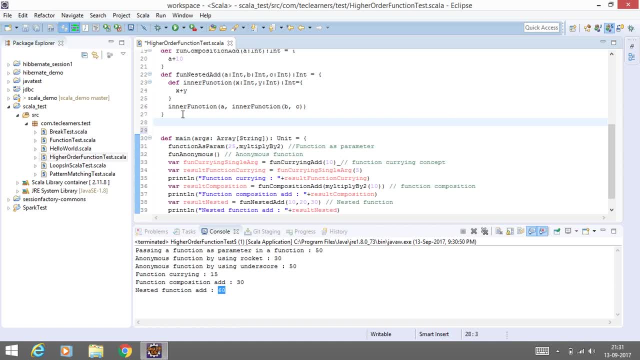 Where you have variable length of data, So variable length of input And you can perform some output. Let's say, make a function Def on variable length. Yes, And I am putting in Integer type of data. Integer type of data. 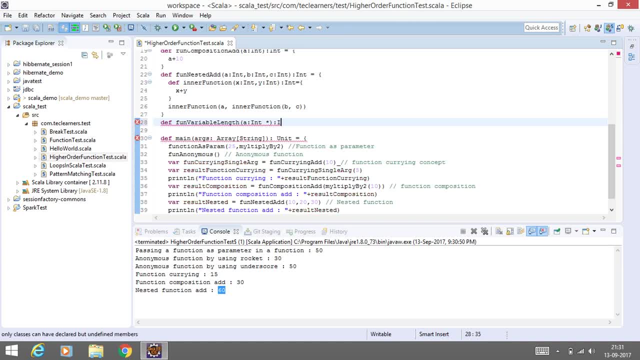 Respective of the number And To return integer type of data. So I will. Whatever the Number of variable input That will be given to this function, It is irrespectively Due to the addition of Each and every number. 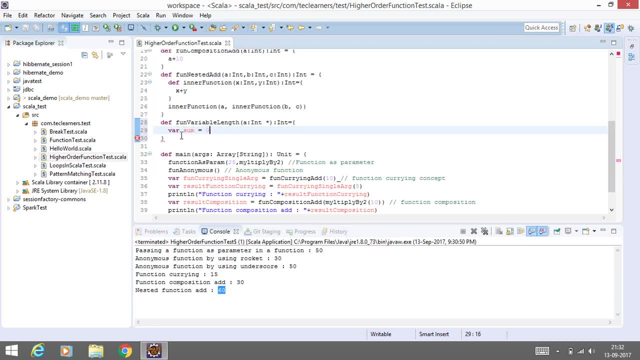 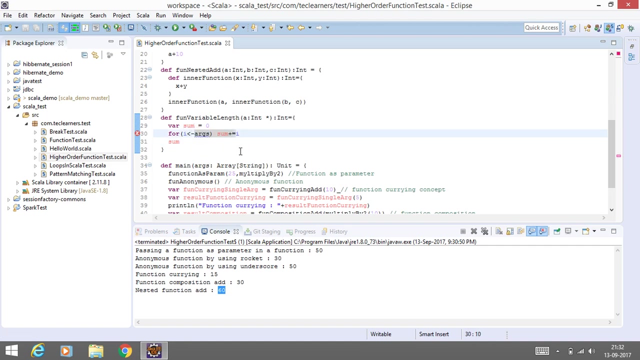 So So The number Given to it, So For I Use Some I And It will return Some. What happens Also? Sorry, I have Put this. I'm sorry I forgot.